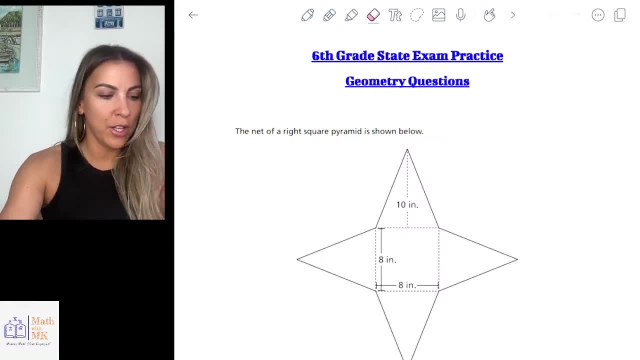 All right, Welcome to the state exam review series. We're going to start with some sixth grade state exam practice questions. These are all going to be questions that are on a previous New York state exam for sixth grade And I'm going to start with some geometry questions and 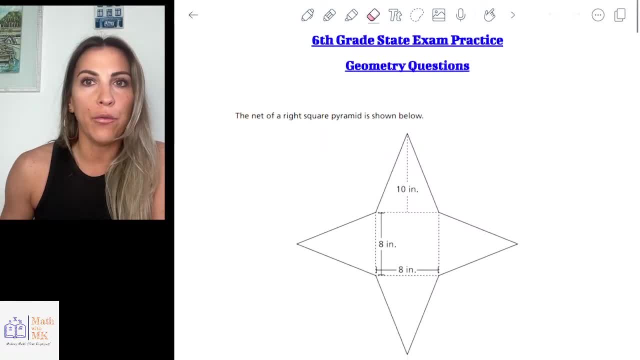 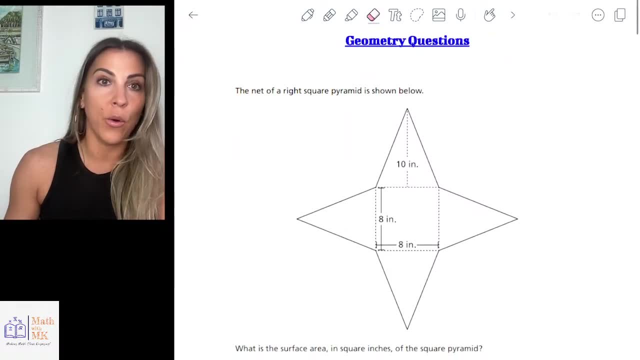 then, um, every week we'll go into some different topics, All right, So if you are not watching this as the live stream, if you're watching a re-recording of this, I suggest that you pause the video and try the questions that are on the screen before I share the answers, so that 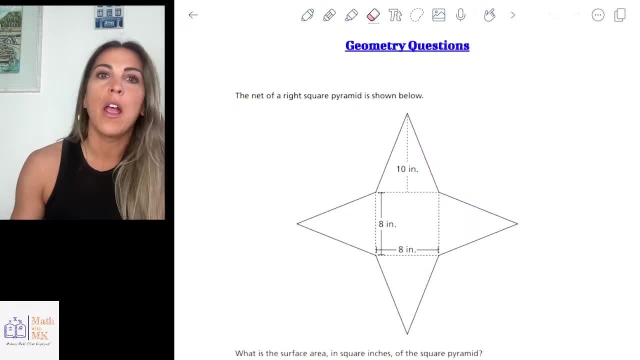 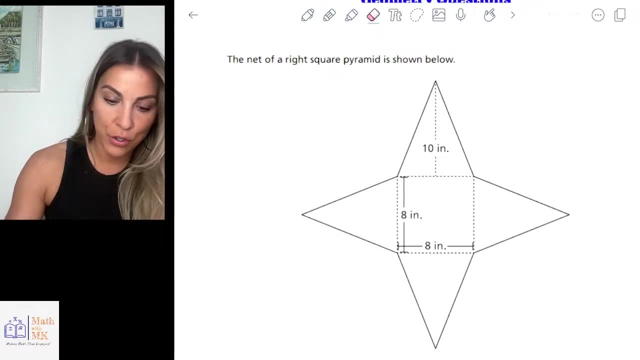 you know whether or not you would have gotten them correct. All right, So let's get started. First question gives us the net of a right square pyramid And the question is asking us to find the surface area of this net of this pyramid, Sorry. So what we need to know is that surface area. 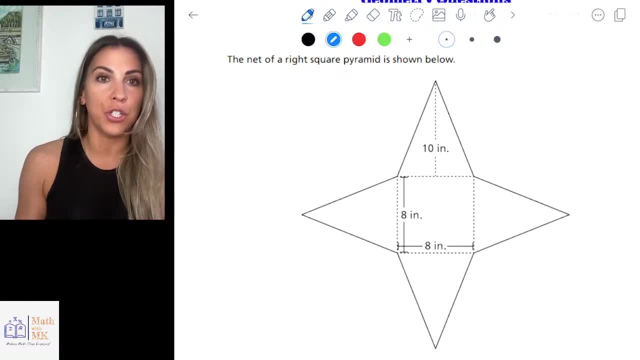 asks us to find the area of each of the faces of the shape that we're dealing with and then add them all together. All right, So when I look at this shape, I see that there are five faces. There's the one square that's in the middle, And then there's the four triangles that 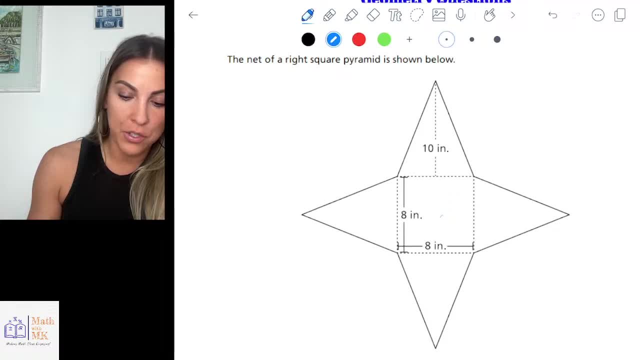 are on the outside. So we need two formulas here. We need to know that the area of a square, that part, is going to be length times width. So we'll find this area first. So the squares length and width of course are the same because it's a square. 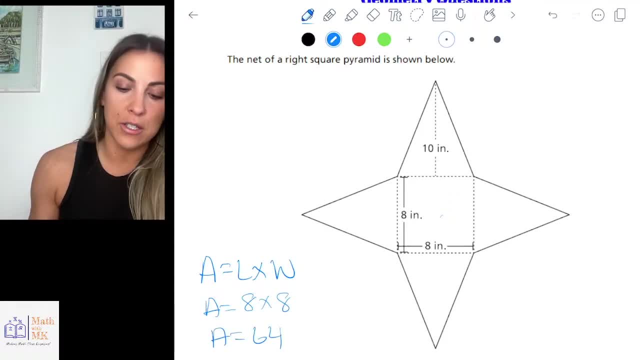 So that area is going to be 64 inches squared, So I'm going to go ahead and write that in here. 64 is the area of that part. So now I need the area of the other four triangles, because this is a square pyramid. I know that they are all the same, So as long as I find the area of one, 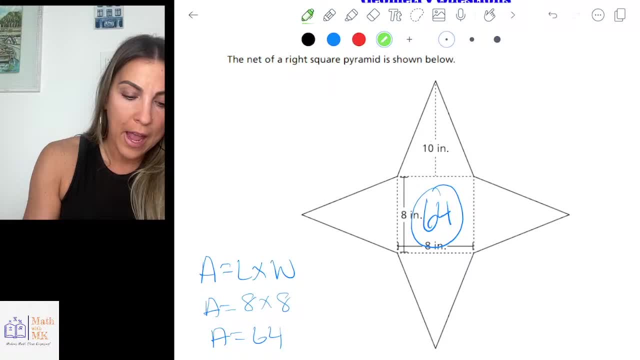 I've got the area of all four, So now I need a different formula, And the formula for the area of a triangle is one half times the base times the height. That formula is on your reference sheet on the test, So use that reference sheet. There's not a lot of formulas on there, but I believe. 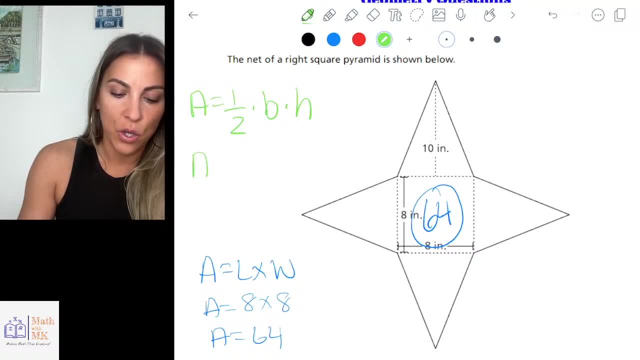 that one's on there. So now it's just about substituting in. All right, So we have area equals one half. We're going to substitute in our base. So the base of our triangle labeled here, this green line, is my base for this top triangle, Even though it's not labeled. 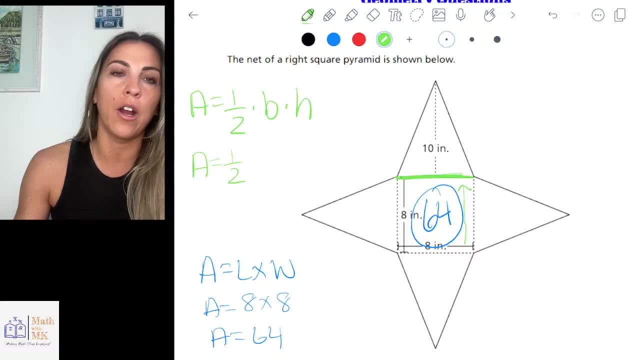 you see that if I took like an elevator up from the bottom of this square, those two lengths are the same. So the base of this triangle is the same as the side length of that square that's right below it. So that's going to be eight, And then the height of the triangle is given to us. 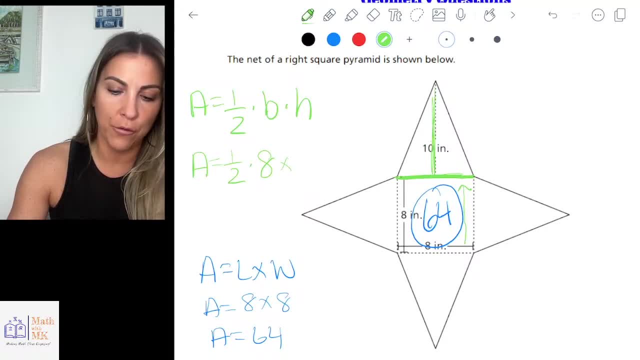 right here, where the height and the base have to be perpendicular, So we wouldn't be looking for this, this side length here, right, We're always looking for the that gives us a perpendicular relationship with the base, And so that's 10.. All right, And so now? 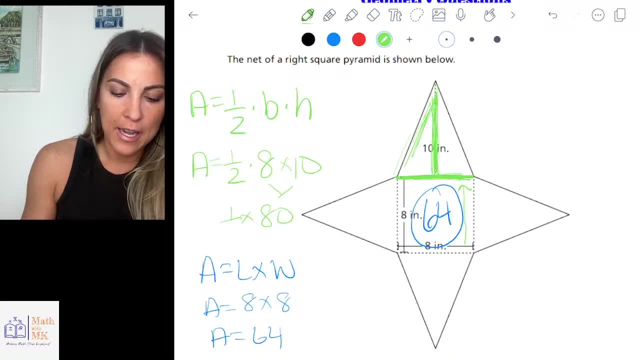 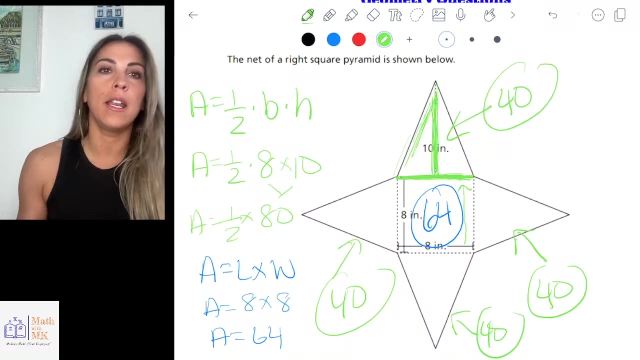 I just have to evaluate. So eight times 10 is 80, and 80 times one half is 40. So that means the area of this triangle is 40 inches squared, And that tells me that the area of all of these triangles is 40 inches squared. All right, And then from the beginning we said that the surface 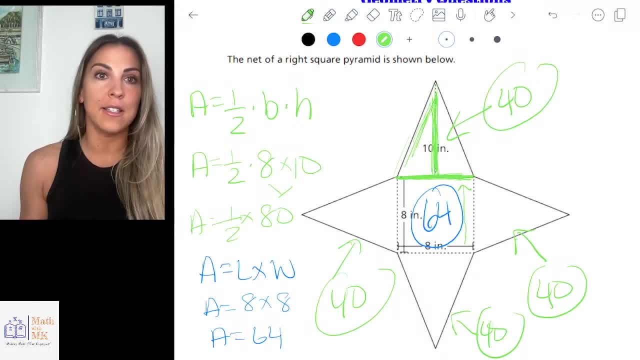 area means you're just taking the area of each of the faces that made up that shape, and we're So. when I think about surface area, I think about gift wrapping. right, You want to cover the surface of each side of that gift, So you need to know how much wrapping paper for the top. 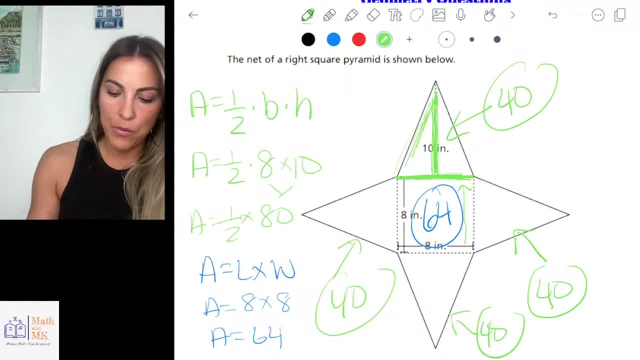 for the sides, for the bottom. you want to cover it all. So if we add all these numbers together, 64 plus, I'm going to write it as four times 40, right, Because there's four equal triangles that are a 40 each. So I get four times 40 is 160 plus 64. And that gives me an answer of. 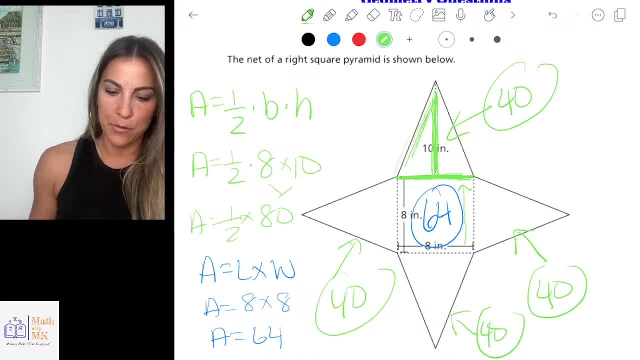 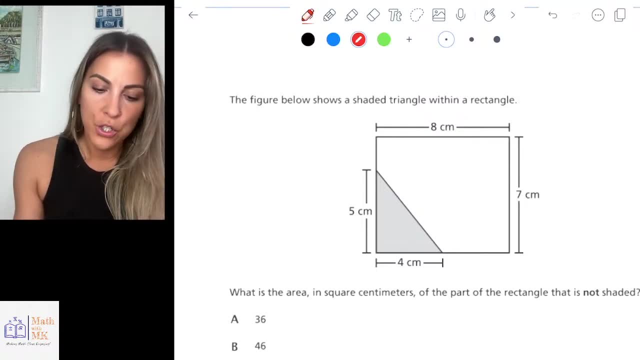 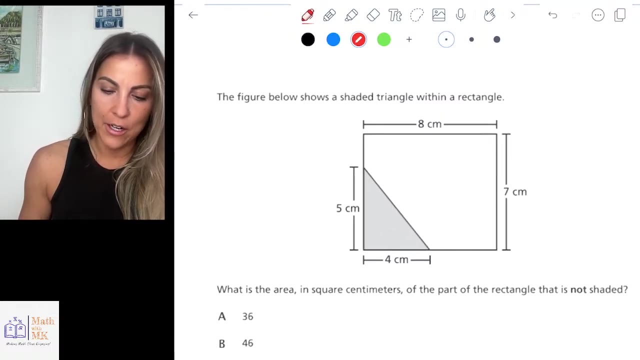 224 square inches for this problem. All right, Let's move on. We're sticking with geometry. This problem says: the figure below shows a shaded triangle within a rectangle. What is the area in square centimeters of the part of the rectangle that is not shaded? So the part in question. 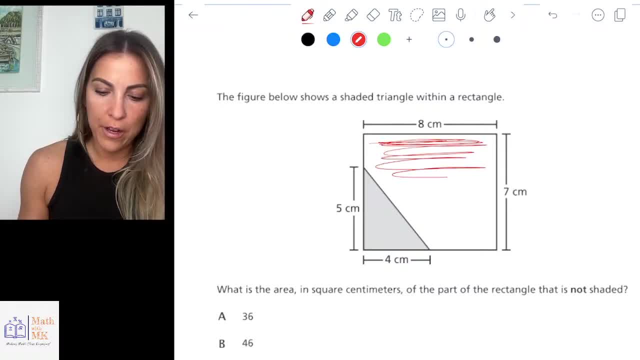 I'm going to go ahead and just shade it in red. They want to know the area of this red piece of this shape. Okay, The area, the part of the rectangle that is not shaded, is the area of the rectangle, The rectangle that is not shaded in. So now you may or may not know how to find the area of this. 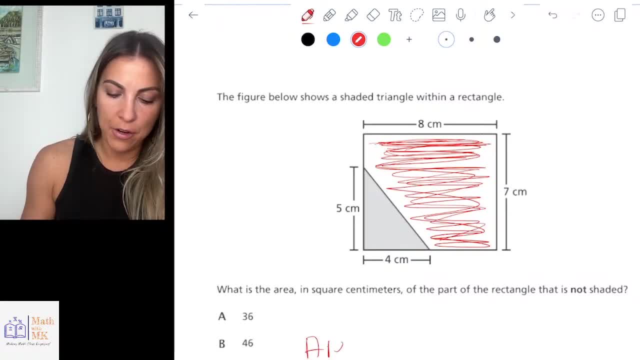 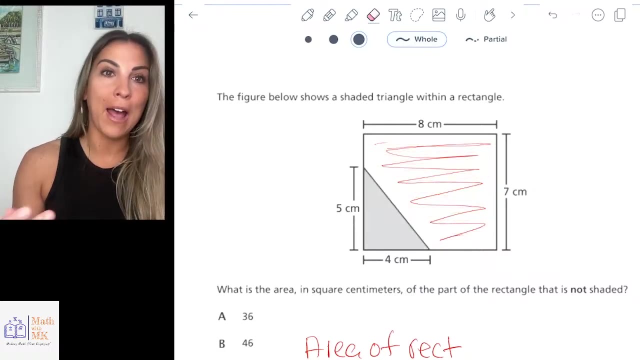 shape. but one thing we can do is we can take the area of the rectangle, not a square. And if I knew the area of that whole rectangle now imagine if they're asking me for only the red part. that means they kind of want us to pretend that triangle isn't even there, right? So in math, 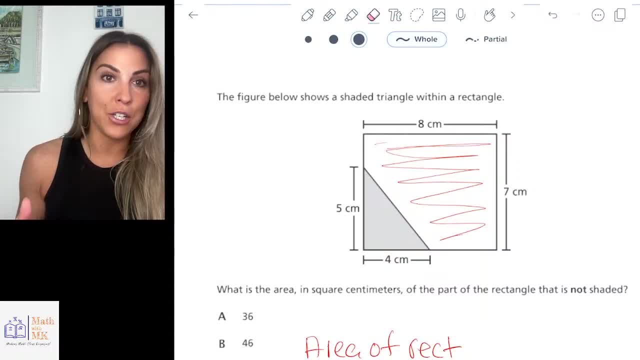 if you're taking something away, that means that the operation is subtraction. So what I'm really doing is finding the area of that rectangle and then I'm subtracting the area of the triangle And that would leave me with the area of that red part. All right, because I'm taking away that. 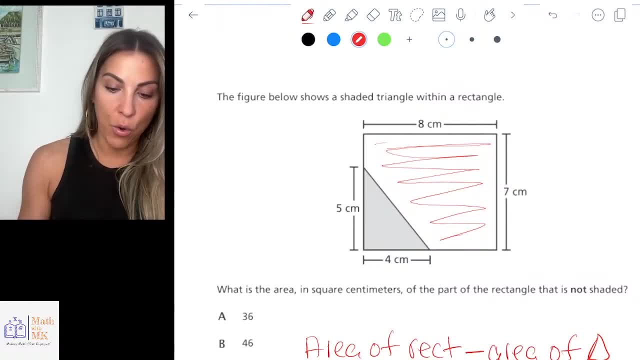 triangle piece from that whole area. So if I find the area of the whole rectangle, let's use a different color for that. So the area of the rectangle is going to be eight times seven right, The length times the width. So the area of the rectangle is going to be 56 centimeters squared. So now that 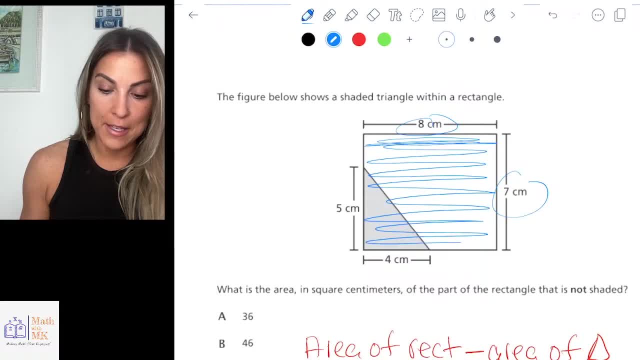 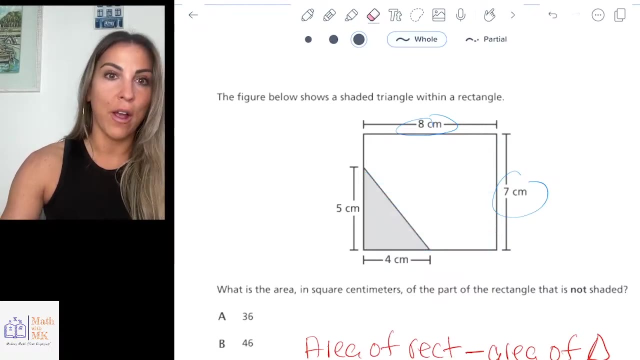 256, that encompasses this entire piece that I'm shading in blue right now. right, The eight times seven means that I'm finding the area of this entire blue piece, But the problem is saying I want to know what the areas of that blue minus this triangle part. That's why I'm going to 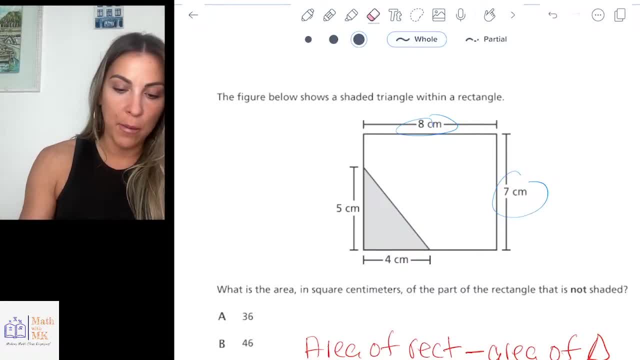 subtract the area of that triangle. So the area of the triangle, like the problem that we just did before. we know that the formula we need is one half times base times height. So I have a base of four right here for the triangle. So one half times four times my height is five. Now we're 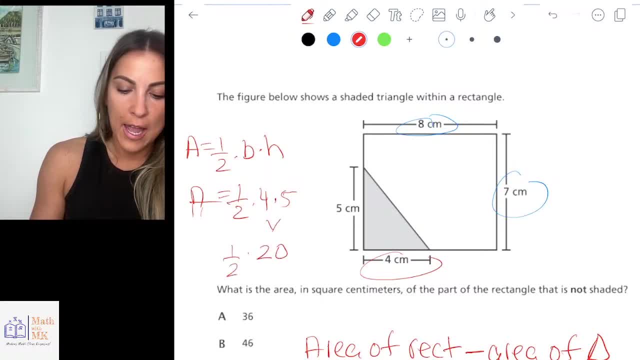 just evaluating again. So four times five is 20 and 20 times one half is 10.. So the area of that triangular portion of this problem is 10.. And we said that we're going to subtract that from the area of the rectangle. So we're going to subtract that from the area of the rectangle, So we're 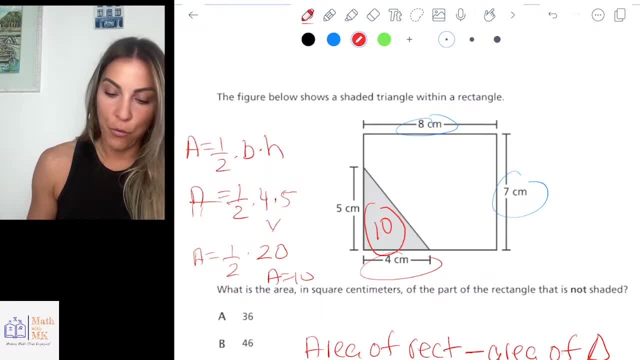 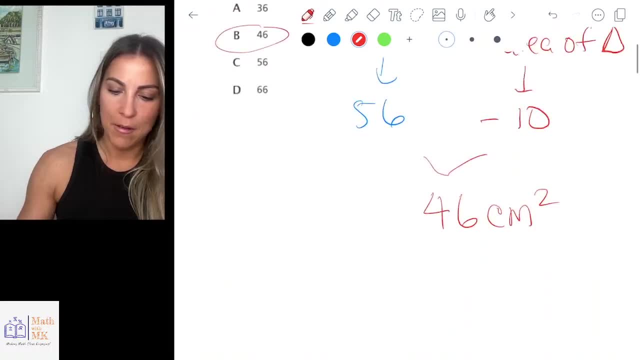 going to subtract that from the area of the rectangle. So we're going to subtract that from the rectangle and that leaves us with a total area of 46 centimeters squared, even though they didn't write it like that in the choices, but they should have. Okay, All right, Moving on sticking to. 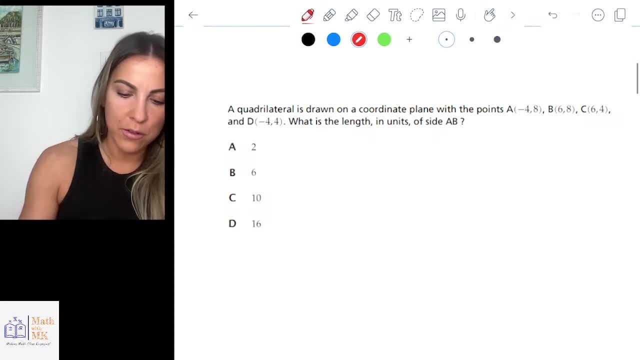 geometry, a quadrilateral. So a quadrilateral is a shape that has four sides. that prefix quad always means four. A quadrilateral is drawn on a coordinate plane. Coordinate plane is just a fancy word for a graph- right X, Y axis with the points A, B and C. sorry, A, B, C and D. 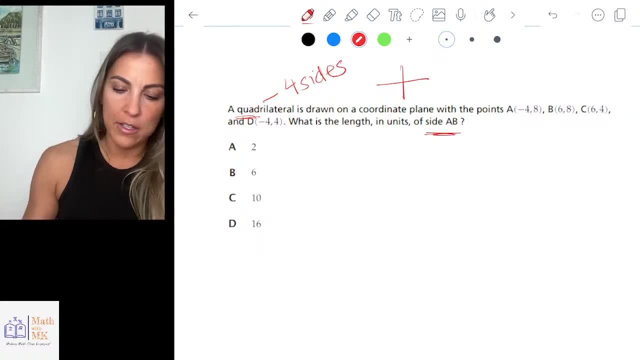 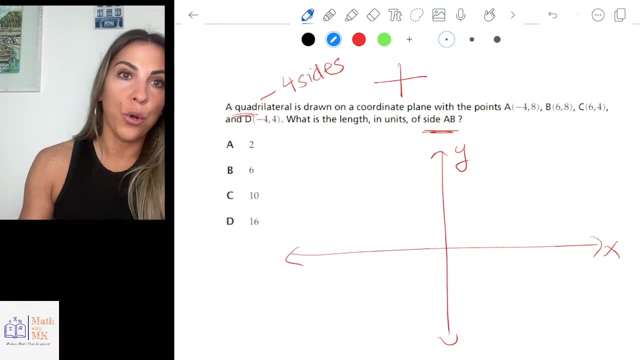 What is the length in units of side A, B? All right, So let's sketch this out. Here's my X axis, The vertical one is my Y axis, And now we have to know how to plot our points. Okay, So the first point, A, is at negative four eight. So in each order pair, it goes X, Y, X, Y. 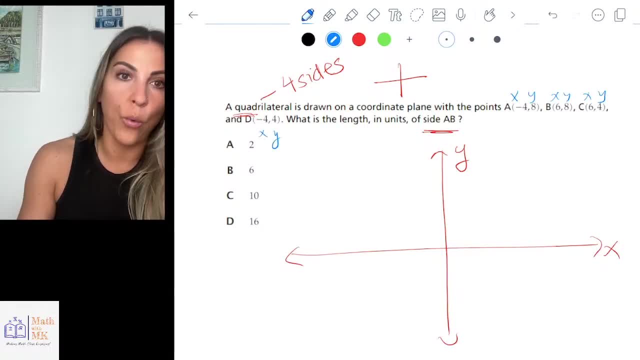 If you forget, it's an alphabetical order, All right. So the X coordinate always comes first. So the X coordinate tells us how much we're going to move and which direction we're going to move on that X axis, on that horizontal axis. So my first X is: 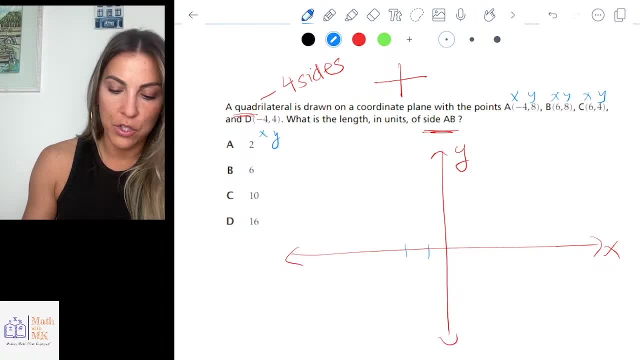 negative four. So along the X axis I'm going to go to the left: one, two, three, four spaces. That'll take me to negative four, And then point A has a Y coordinate of eight. So I'm going to go. 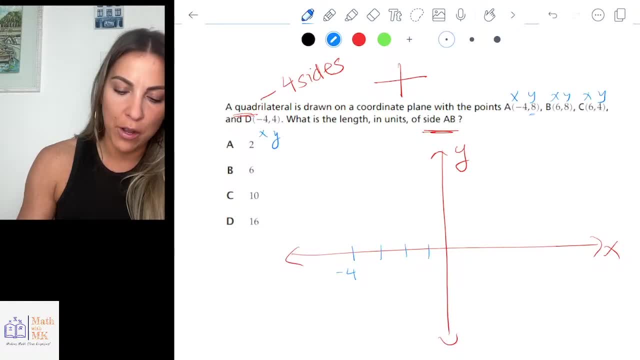 up eight. I'm not going to do this exactly. Obviously I don't have a perfect graph drawn, but I know that eight is going to be somewhere up here and this is clearly not drawn to scale. It should be higher, but that's not going to happen, So I'm going to go up eight. 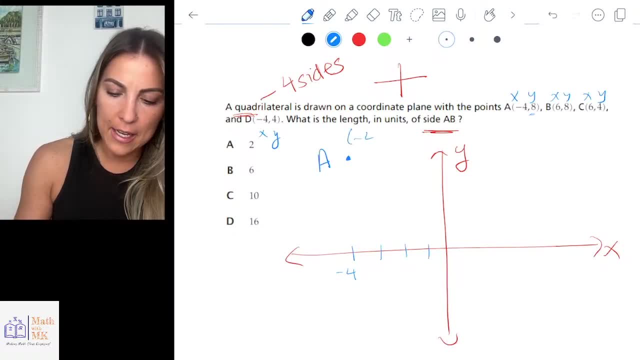 Okay, So we're going to label this point A and that's at negative four eight. Moving on to point B, B is going to be at six, So that's a positive number for the X. So now I'm going to the right side of the origin, this dot in the middle that I'm labeling right now. That's my. 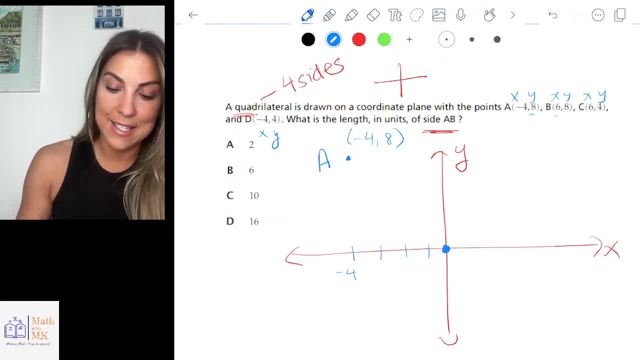 origin. That's the point, zero, zero. So now B is six, eight. that X coordinate is six. So I'm going one, two, three, four, five, six, again not drawn to scale, but you don't have to worry about it. 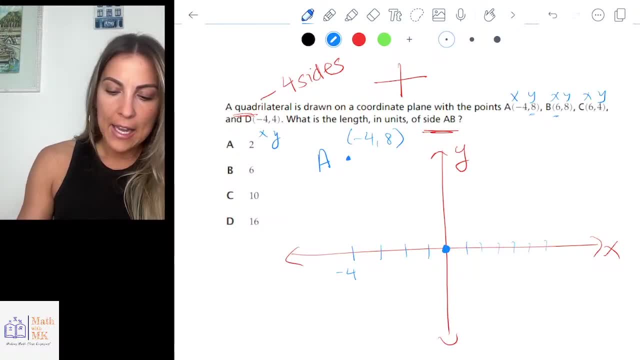 And you'll see why in a second. And then my Y coordinate is eight, And even though this isn't drawn to scale, what I'm going to do is try to go up about the same amount that I did for point A, because their Y coordinates are the same right. So negative four, eight, six, eight, even though 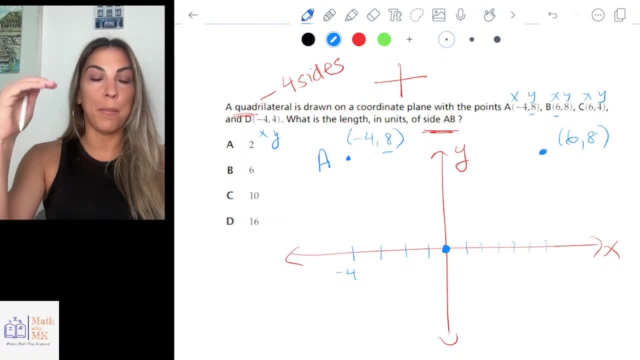 they went in different directions. horizontally they both went the same amount up. So if you picture that Y axis as an elevator, both points A and B took that elevator eight flights up. So they stopped at eight. So they should be in line there, All right. Moving on, point C is at six. 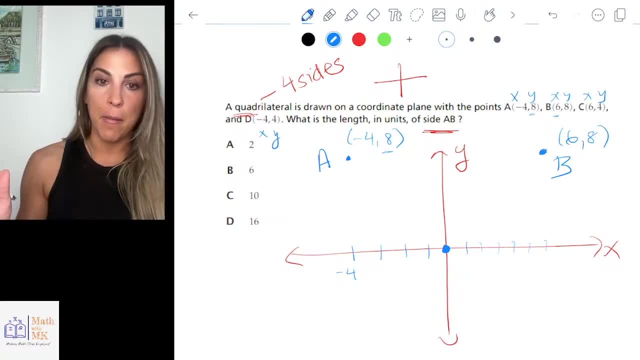 four. So for C, now I'm going over the same amount for B. right, It went over six as well, but now I'm going up only four. So about halfway there, or exactly halfway there, I should say All right. So that's point C. 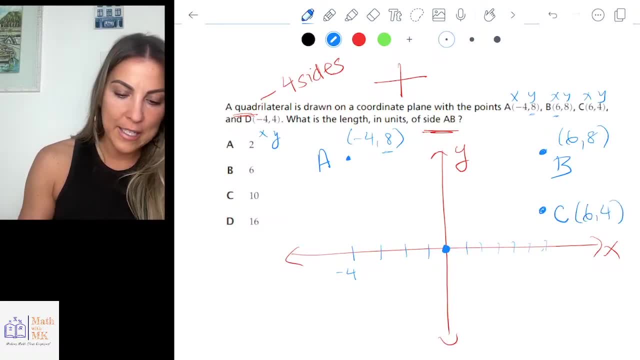 which is going to be at six four. And lastly, I have point D which is at negative four, four. So negative four is my X coordinate. So we said the X coordinates that's going to be my horizontal axis And if they're negative we're going to the left of the origin. So I'm going negative four. 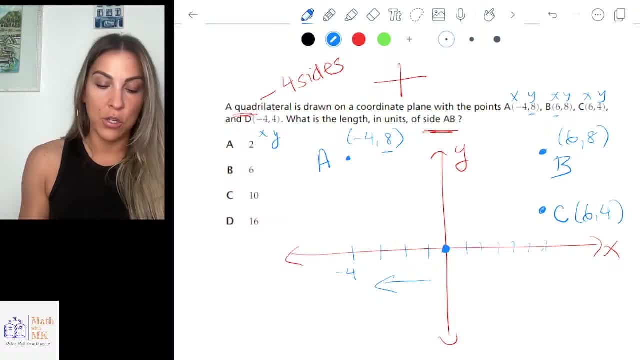 which is exactly how far left I went for point A. So I'm going to make sure that's in line and then up four. So again halfway up, All right, And I'm going to connect these to make the rectangle that they're talking about. Well, they didn't say. 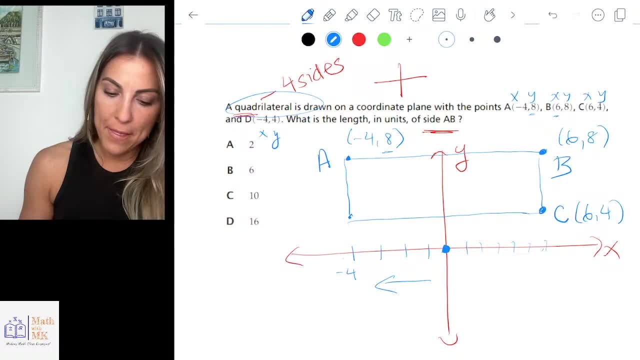 rectangle- They said quadrilateral, but it is a rectangle, All right- And they want to know what the length is of side AB. So they are looking for the length of this green line right here Now, because A and B have the same Y coordinate. all I need to do is count the distance. 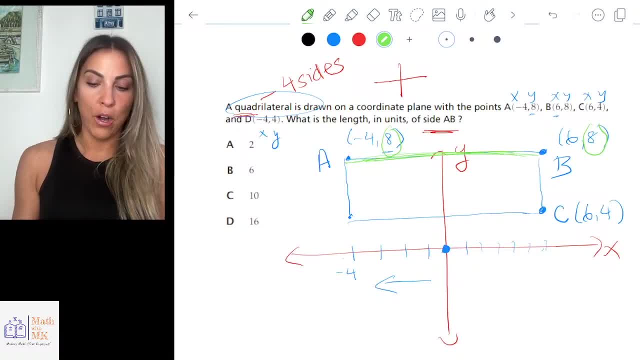 between their X coordinates. So how far is negative four from positive six? All right, So from negative four to zero, which would get me to the axis, that would be four spaces, And then to get from zero over here to six, that'd be another six spaces. So that means that I have 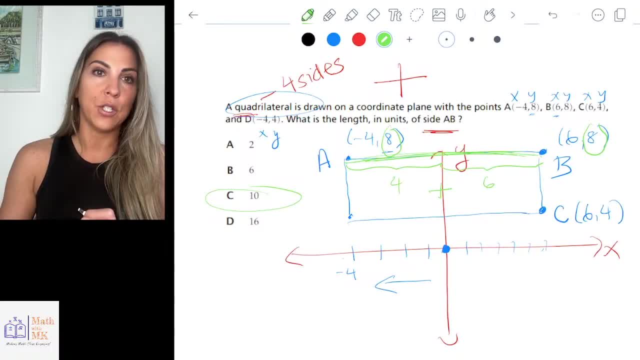 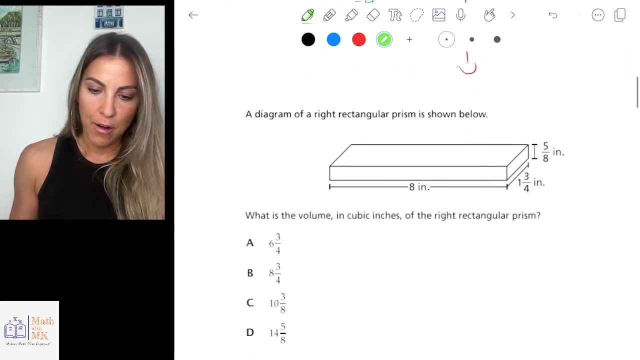 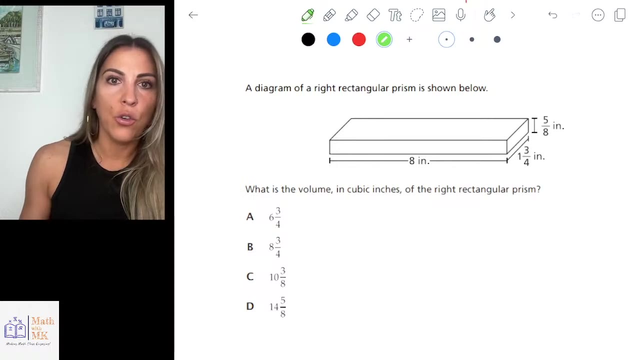 four plus six, a total of 10 spaces that I have to travel. So the length of side AB is going to be 10 units. All right, Sticking in geometry, I'm going to start moving on to a volume problem. So they want to know the volume in cubic inches. 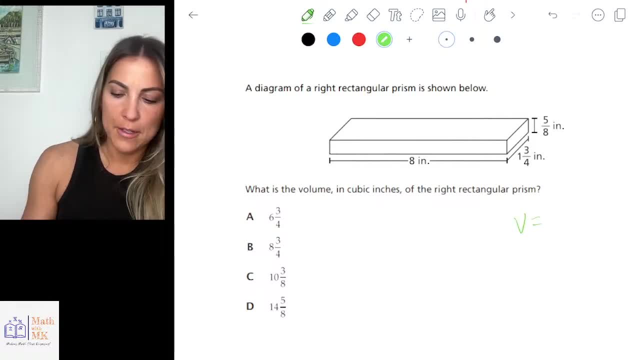 of the rectangular prism. So volume- the formula for volume is going to be base times, width, times, height. The problem, the tricky part about this problem, is that they also put fractions in there. So you have to know the formula for volume. You also have to know how to multiply fractions. 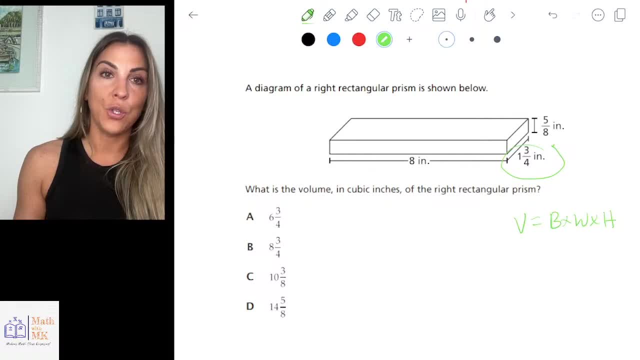 All right. So the first thing I'm going to do is change this mix number over here: improper fraction. So if you need a review of that, I'm going to bring that over here to the left: one and three fourths: I want to make that a a improper fraction. So to make it an improper. 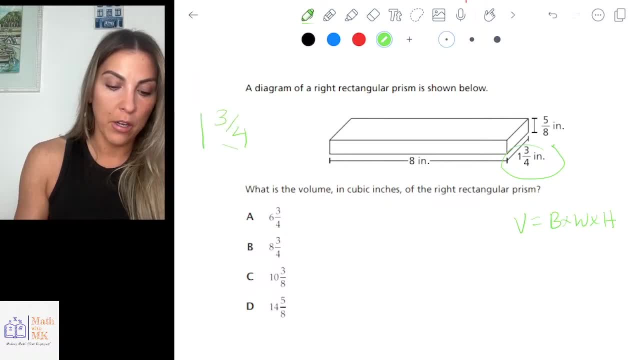 fraction. you multiply the denominator by the whole number. So four times one is four, And then you add that to the numerator. So four times one is four plus three is seven, And I keep that denominator of four. So one and three fourths is the same thing as seven fourths. Okay, And to do? 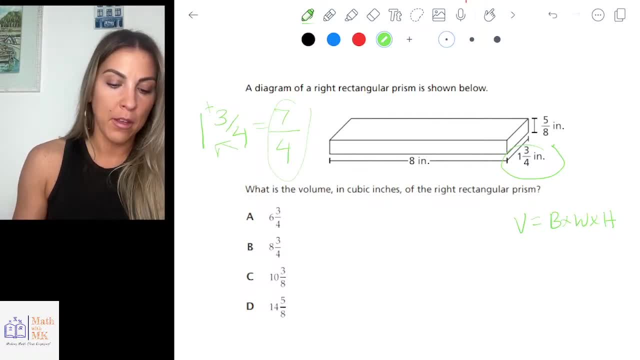 a quick check, four goes into seven one time, and there's three left over, So three out of four, right? So I'm going to rewrite this guy as seven fourths of an inch before I substitute in. So now to find my volume, I'm multiplying eight times five over eight times seven over four. All right, 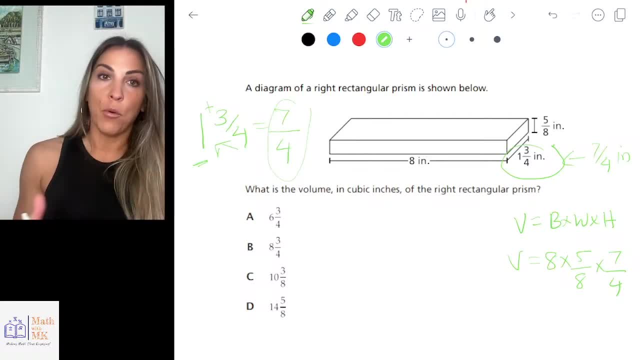 Now you can multiply fractions um in the most straightforward way, which is to multiply numerator times numerator, in this case times numerator, because we have three of them, And then denominator times denominator, Nominator times denominator. And there's your answer, And it probably has to be simplified. 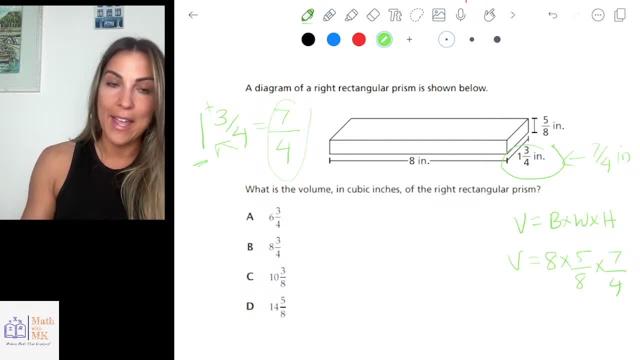 Um, but what I always like to check for is to see if there's any shortcuts. So if any of the denominators can be divided into any of the numerators, I can simplify that first, So I can see that this eight goes into eight one time. So that wipes that part out for me. So now all I have 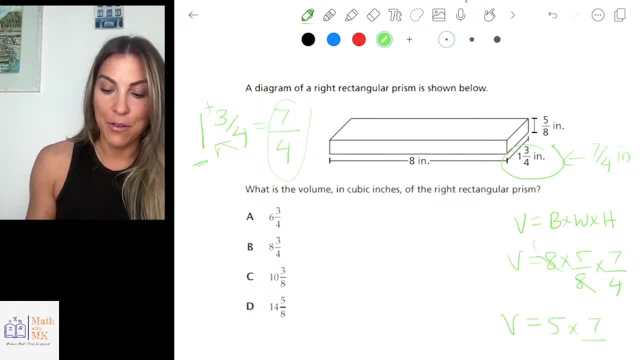 left to multiply is five times seven over four. five is the same thing as five over one, because fractions are division. So five divided by one is still five. So I haven't changed that. So I'm really just doing five over one times seven over four, And then again to multiply fractions. 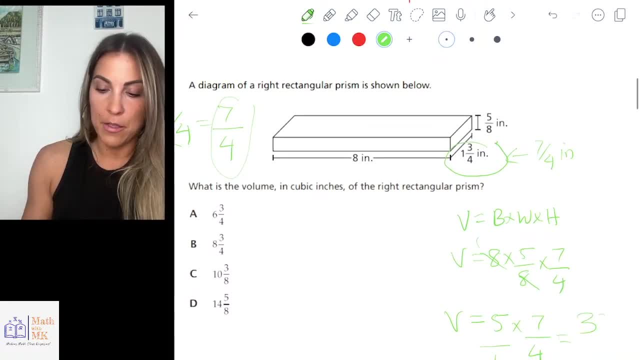 you go: numerator times numerator. So five times seven gives me 35 over denominator times denominator. So one times four gives me four. So now my answer is 35 over four. but the tricky thing about multiple choice problems is, if you look over here I don't see 35 over four as an. 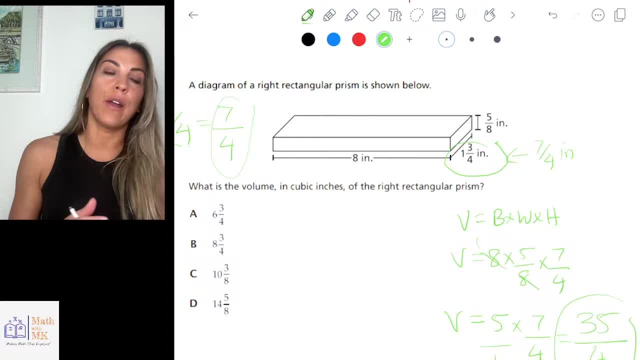 answer. So this is why knowing different versions of how to write a express a number in different ways, is important. So 35 over four can be written as a division. So I'm going to do that, So I'm going to go into decimal. It can be written as a mixed number. I see that my answer. choices are all in. 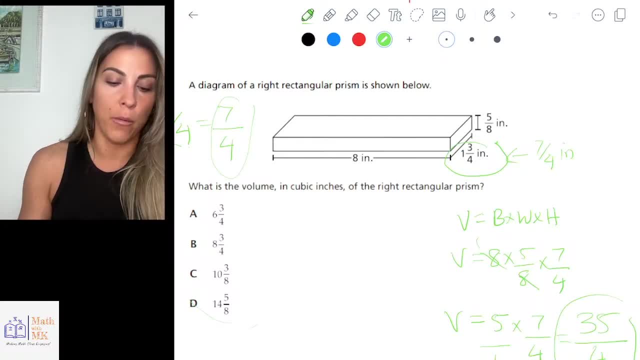 mixed numbers, So I need to know how to convert this. All right, So we're going to go backwards from what we did up here. So four goes into 35,. eight times eight times four is 32.. And that leaves me three left over. So I have three left over out of four. So 35 over four is the same. 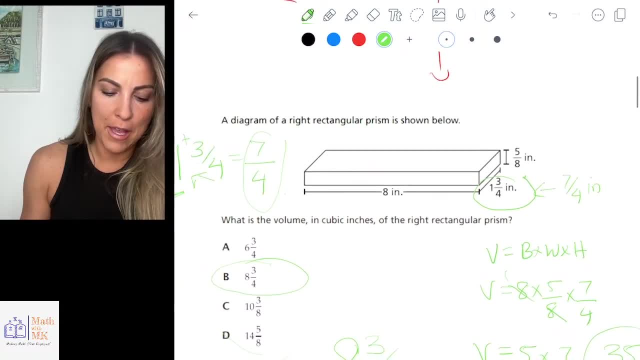 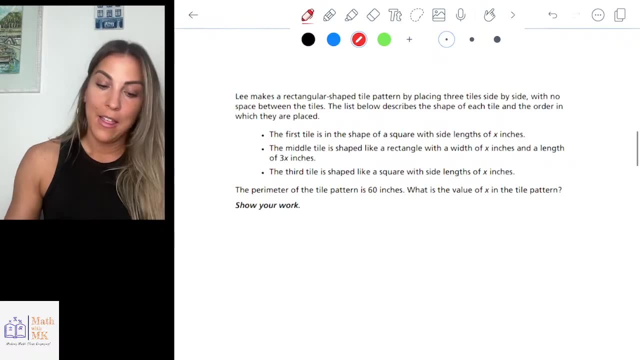 thing as eight and three fourths, which means that answer choice B is going to be our answer for this volume problem. All right, We have two more Geometry problems. This one is a lot of words and no pictures, And my advice to you is to always 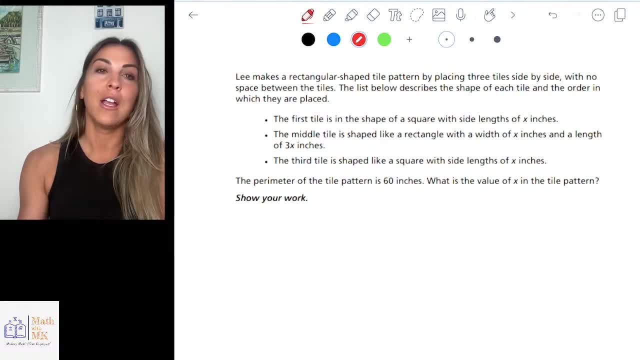 try to draw something when you get these problems, because it can be really hard to imagine what's going on without picturing it. So Lee makes every tangular shaped tile pattern by placing three tiles side by side with no space in between. All right, So we got three rectangles, or sorry, it's going. 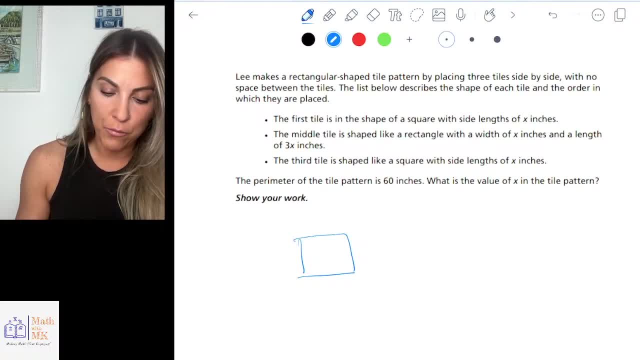 to be a rectangular shaped tile pattern, And we're going to show three tiles with no space, So you're going to be able to see how the two of them are connected. right, That helps me visualize what's going on in this problem. The first tile is in the shape of a square with side lens of X. 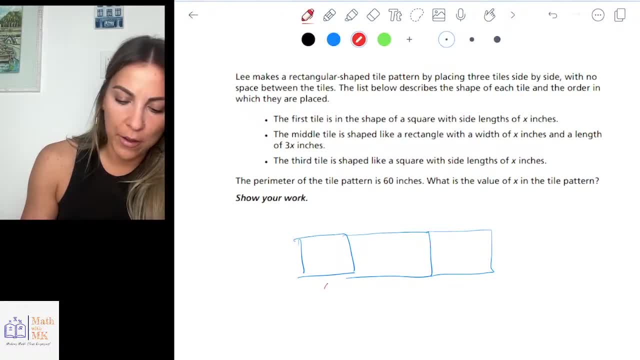 inches. So we know that a square has lens that are the same size. So if I label this X, then I know that this is X and this is X and this is X. So that's that first square that they're talking about right here in that bullet. The middle tile is shaped like a rectangle with a width of X. 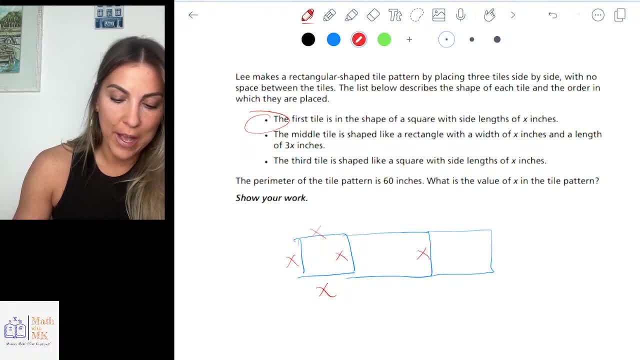 inches. So of course it actually has to have a width of X inches because they were attached. So that's that width that it shares with the square. And then this one is of course also X, because it's a rectangle, and a length of three X inches. So I already knew that, which is why I drew this longer. 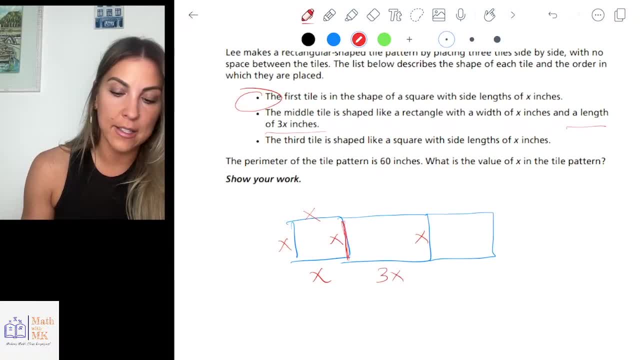 but if you hadn't, you would erase it and draw longer. Now this is three X, So the length of that rectangle is three X. We know that a rectangle has the same length and the same width, So if that's three X, this top part is also three X. I don't know if I'm going to need. 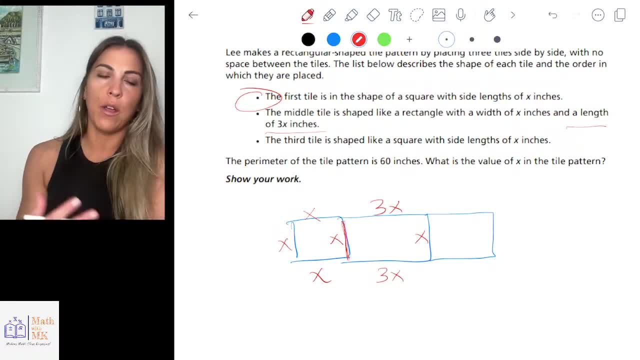 all these labels, but I'm labeling now my picture so that I can see what I'm working with And then I can determine which of this information I need. So that's that second bullet. We finished that. And then the third bullet says the third tile is shaped like a square with side lengths of X. 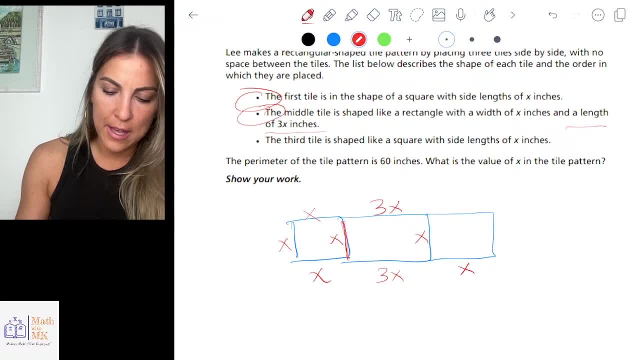 inches, So that last tile looks exactly like the first one, where it's X, X and X. All right, So we have our picture drawn. We know what we're dealing with. Now let's find out what they want. The question says the perimeter of the tile is 60 inches. I'm going to annotate that word: perimeter. 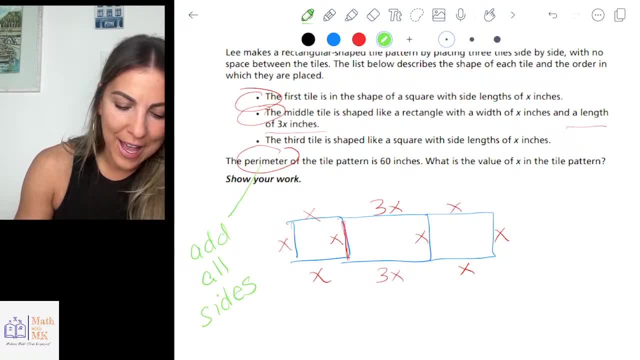 Perimeter means to add all the sides On the outside, So the perimeter is the outside of a shape. The perimeter is always those fence problems. that asks us how much fencing we need, Cause you put a fence on the outside of something. Okay, So it has nothing to do with the inside parts and it's going to be 60 inches. So when I 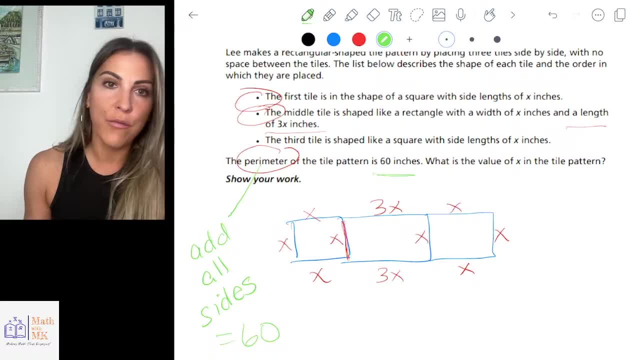 add up all those sides, I'm supposed to get 60 inches. What's the value of X? All right, So now we're going to set up an equation to solve this. Now just to figure out which sides I'm going to be adding up. So the perimeter is the um, the sum of the outsides of this shape. 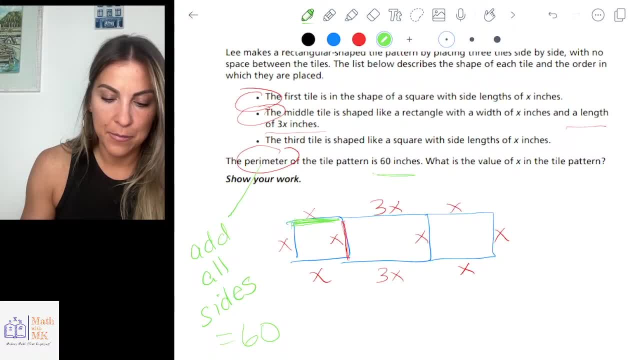 So I have X plus three X plus another X plus another X. So you see how I'm just kind of following a pattern to get around this whole shape: plus another X plus another three X, plus another X plus another X, And that gets us around the whole shape. All right. So even though I knew, 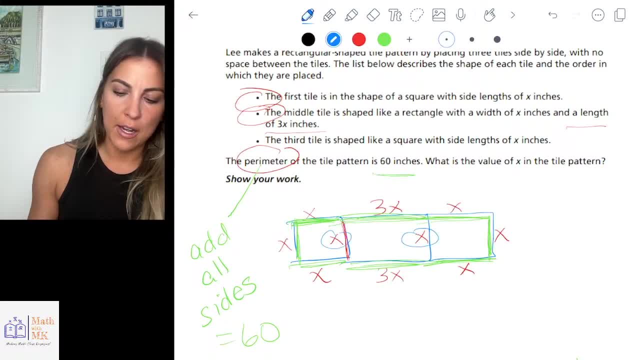 these measurements that I'm circling in blue. those are not important for this problem, because it's asking us about perimeter, which is the outside shape, So I don't need to know that, All right. And now the other fact that I know is that all of this 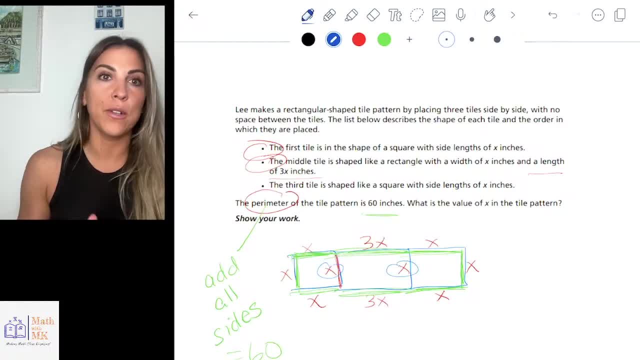 when I add it up, it's supposed to equal to 60, the perimeter is 60. So if I take all those expressions, all those terms, and I add them up, I'm going to get 60.. Having that equal 60 is. 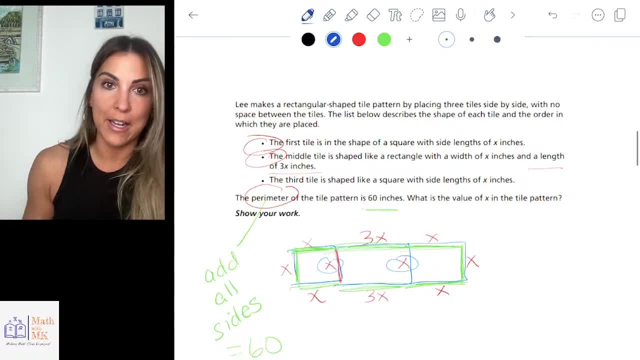 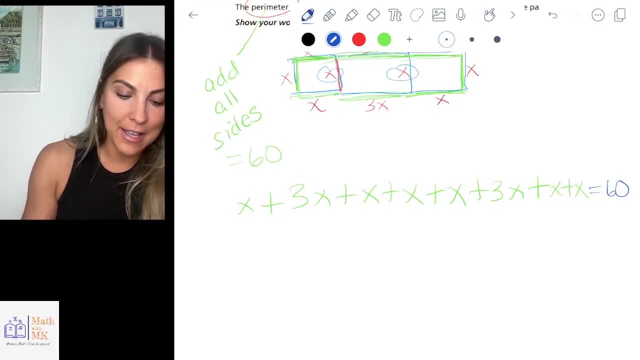 vital and helping me figure out what X is, because now I have an equation that I can solve, So I'm going to start combining all these like terms that I wrote. So I see, remember every X has in front of it and invisible one, as the coefficient anything times one is. 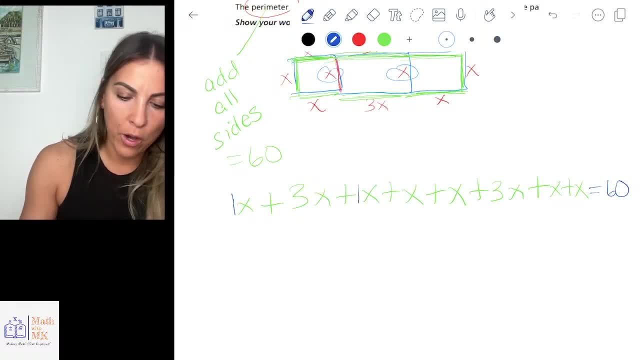 itself. So I don't change it if I put a one in front of it. So I'm going to put a one in front of all of these Xs so that we don't forget them when we're adding. So I have all the same variables. 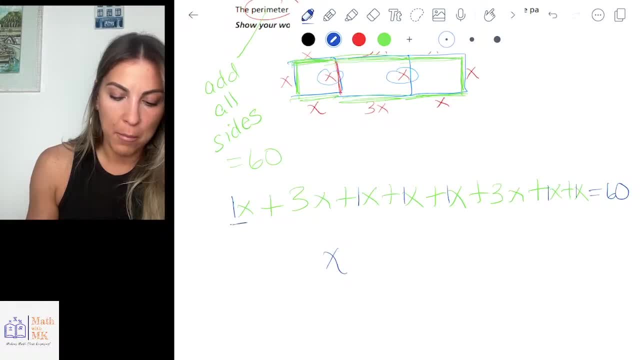 So I'm going to end up with something in front of the X and I'm going to add up one plus three, So I have four, five, six, seven, 10,, 11, and 12.. I have 12 Xs when I add up all those like terms. 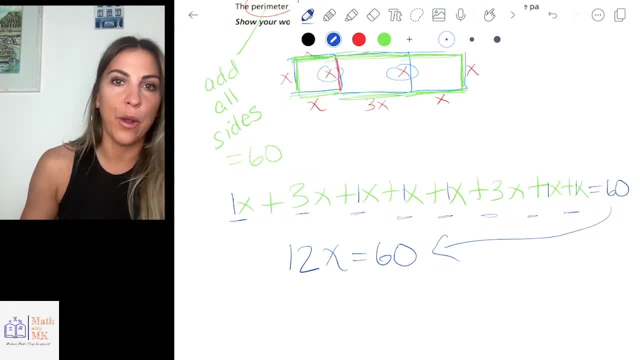 equals 60. Then I'm pulling down from that part of my equation. All right, And now to solve an equation, you do the inverse operation. So it says 12, X equals 60, 12 and X are being multiplied. When you have a coefficient and a variable next to each other, with nothing in between, that means 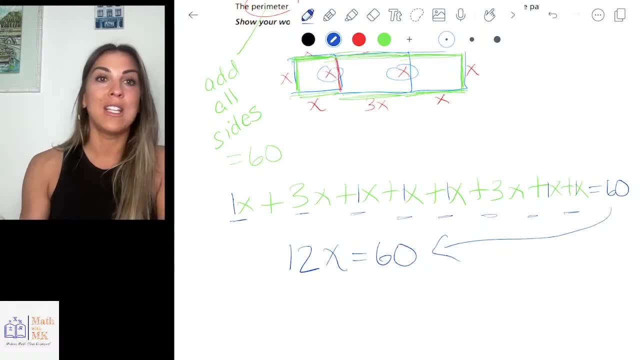 they're being multiplied. So the opposite of multiplying- because we use the inverse or the opposite- is dividing, And I'm going to show dividing by a fraction. So I'm dividing by 12 on both sides. Why am I doing that? Because if I divide by 12, I'm dividing by 12 on both sides. 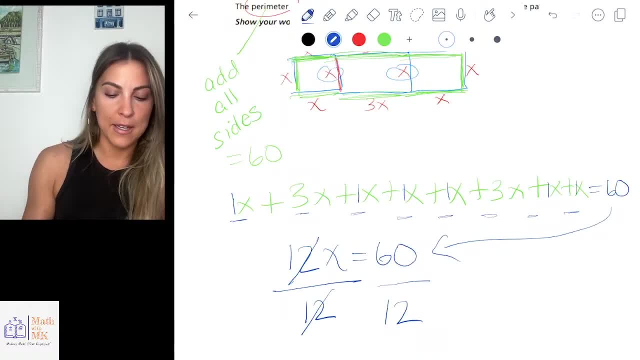 12 by 12 on the left. it'll give me one One times. X is just X. So what did I do? I got X by itself. That's the goal You're trying to get X by itself. So that's why you do the opposite of. 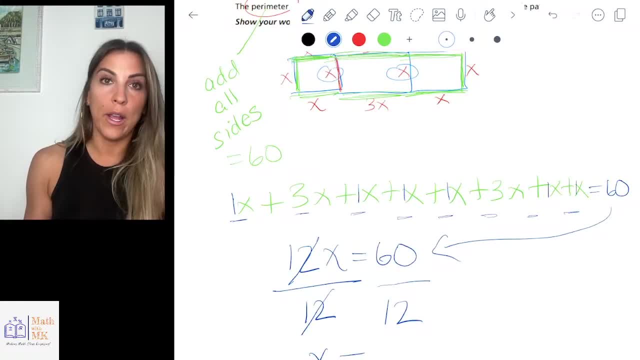 whatever's happening to X And on the right side, because it's an equation: whatever we do to one side, we have to do to the other side to keep it equal. So I do 60 divided by 12, and that gives me. 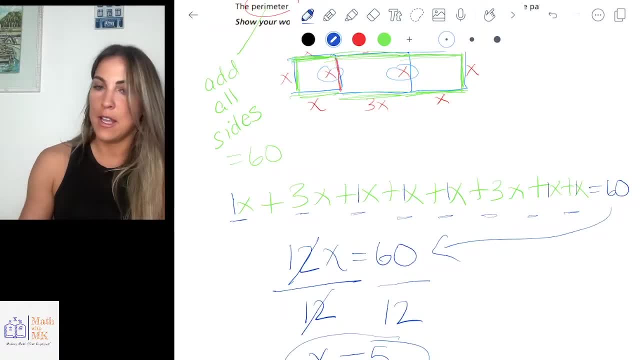 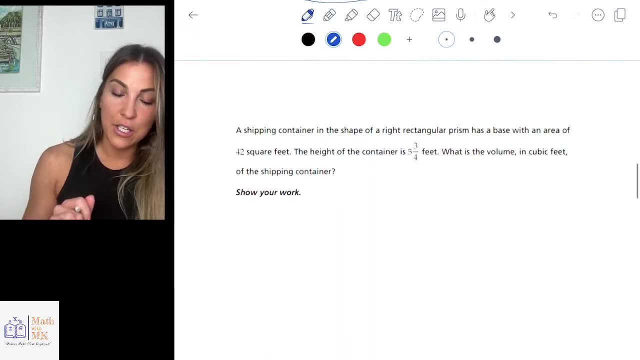 five, So X equals five is the answer to this problem. All right, So this is another one that doesn't have a picture, So we'd be better off trying to draw something for ourselves and helping ourselves visualize it. A shipping container in the shape. 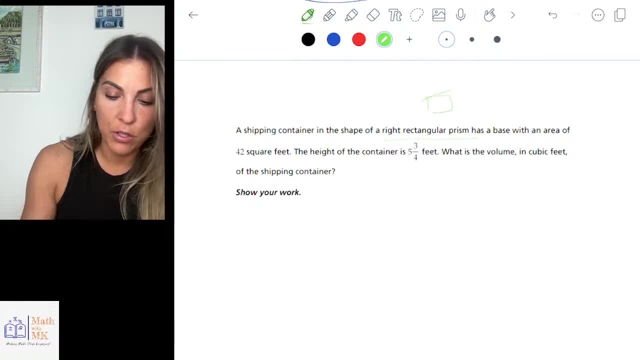 of a right triangle- sorry, right rectangular prism. So we're looking at a shape that looks something like that Has a base with an area of 42 square feet, Okay, So let me make this bigger and see if I can make this look like a right rectangular prism for you. 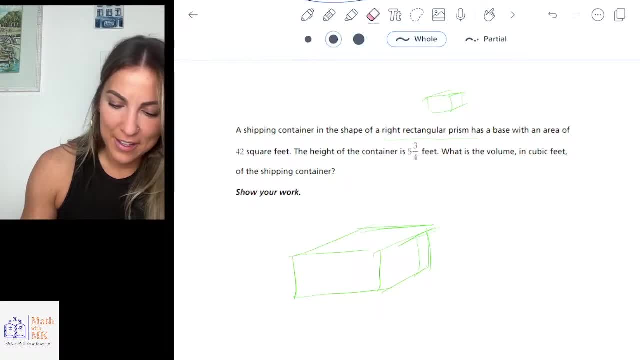 Okay, Something like that, nor this, All right. So let's see the information we have. The height of the container is five and three fourths feet The area of the base. So when we talk about the area of the base, I'm going to kind of draw the inside of this. They're talking: 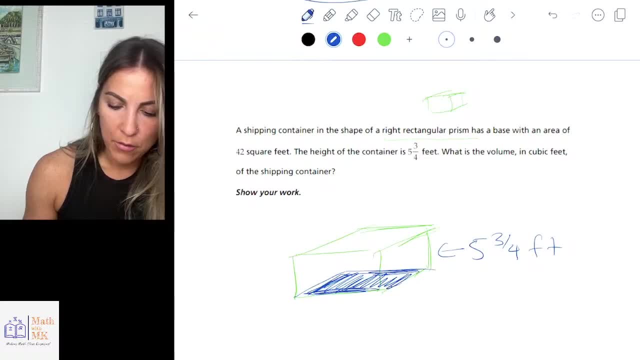 about this blue part of the shape right. So it's not one dimension, It's not the length, It's not the width. They're talking about giving us that whole area, So that area is 42 feet squared, and they want us to find the volume. So the volume for a 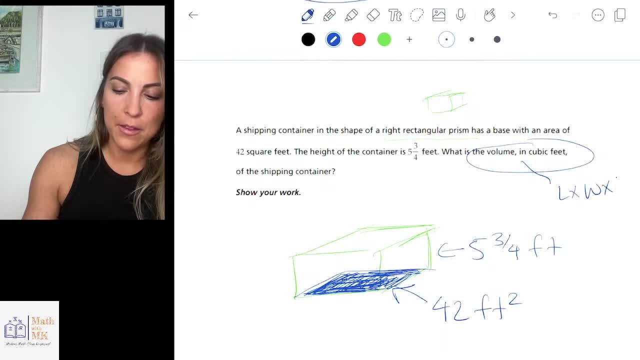 rectangular prism is going to be length times width times height, or base times, width times height, however you want to look at it. So it looks like the formula is requiring us to have three dimensions, but length times width, this first part of the formula. if I multiply the 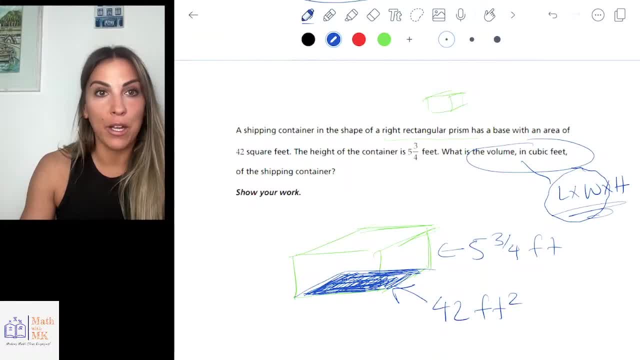 length and the width of a rectangle, I will get its area. So what this probably means is that I'm going to get the length times width times height. So what this problem did for me is actually give me the length times width. That's the 42 right. 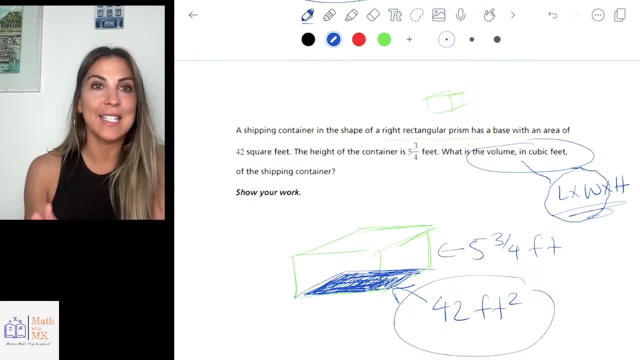 here. So they told me the area. but length times width is area. So when I go to substitute into the volume formula length times width, times height, the length times width is 42 because it's already been multiplied. I don't know what the length and the width are, but I know that when 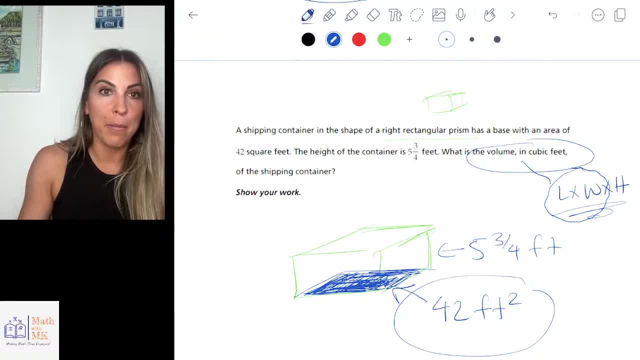 I multiply them I get 42, because that blue part in my picture that's the area. I got that area by doing length times width, So they kind of did that part for me. That's why you'll see on your reference sheet Sometimes the 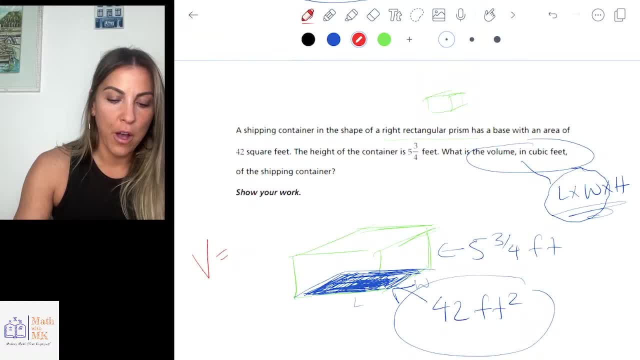 area formula is written in two different ways. It's written as: or sorry- the volume formula. It's written as: capital B times height. That capital B is not base. That capital B means the area of the base. So if you're given the area of the base, you just need to multiply that area. 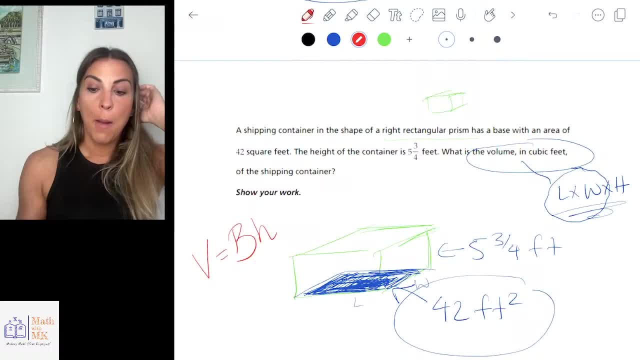 of the base times the height. But if you're given the length, the width and the height, then you would use what I'm boxing in the red over here. You would multiply all three of those dimensions: length times, width, Times, height. All right, So I had 42 already given to me, and then I have five and three. 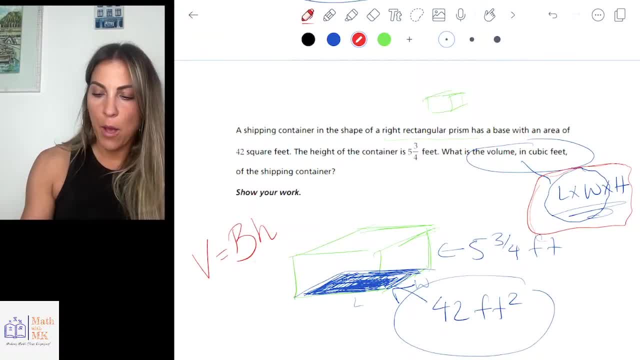 fourths as my height, All right. So just like we did in that problem before, if I'm going to multiply a mixed number by a whole number, I want to change that mixed number into an improper fraction first. So five and three fourths as a reminder how we made it into an improper. 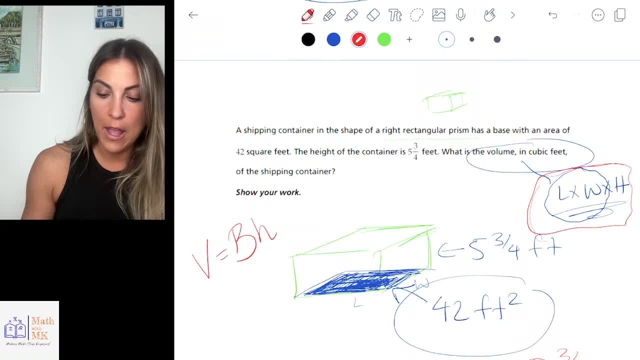 fraction. we multiply the denominator by the whole number. So that gave us 20.. And then we added 20 to get 23.. And we keep the denominator. So 23 over four is the same thing as five and three fourths. Okay, And then I'd be multiplying 42 times 23 over four. All right, Is that right? 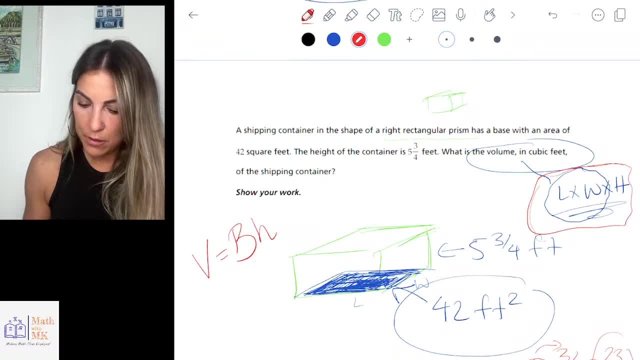 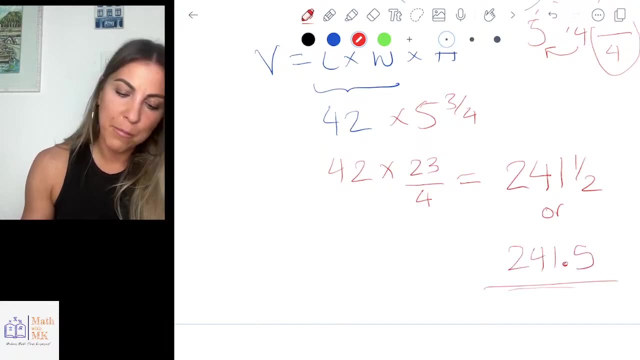 Yes, Okay, And then when we multiply that out, we're going to get 24,, 241 and a half. where are we? Or 241.5.. So again, not important here because it's open-ended, but if it was multiple choice, you always want to know how to express it. 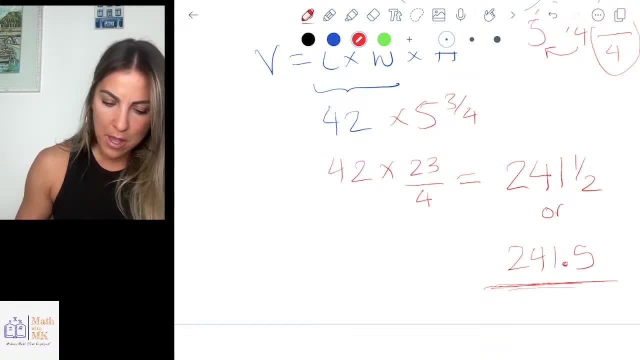 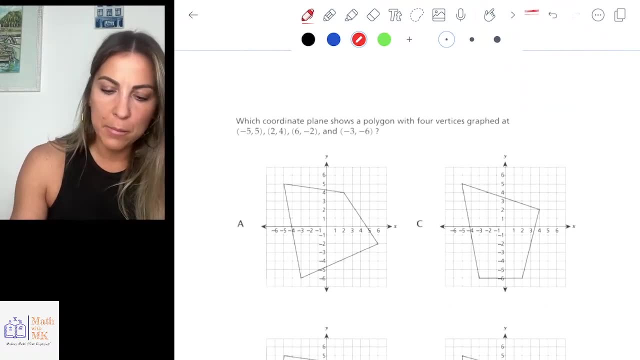 in two different ways, just in case. All right, Let's see We have time for one more geometry problem. So this one is going to be plotting points again. which coordinate plane shows a polygon with four vertices graphed at these points. So, just like we did before we talked, 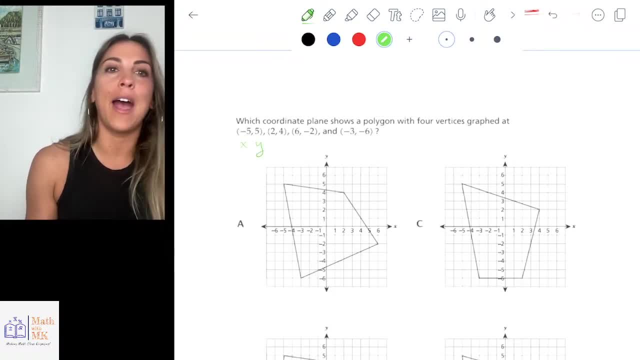 about the fact that every ordered pair has an X and a Y in that coordinate plane. So we're going order. Remember alphabetical order. So X, Y, X, Y, X, Y. We also talked about the fact that the horizontal axis is the X- but in this problem it's labeled for us anyway- And the vertical. 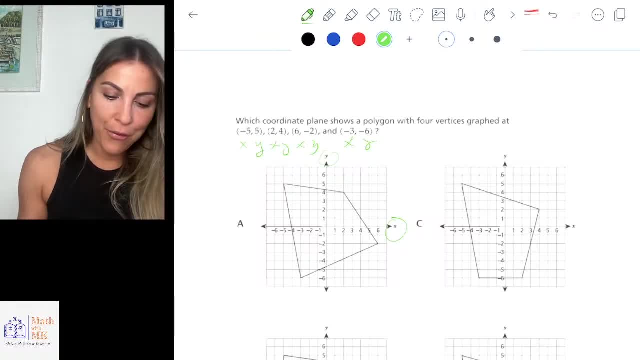 axis is Y, So let's look for that point. Negative five, five negative five is my X coordinate. So on that X axis, on that horizontal axis, I'm going to the left of zero because that's where my negatives are. So I'm going over to negative five on the on the X axis. I'm right here. 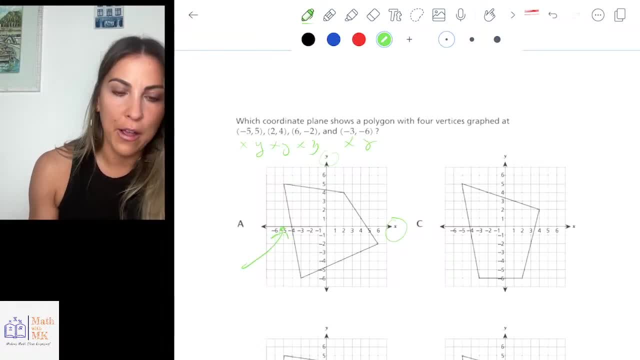 but I'm not plotting that point yet. but I'm right here at negative five. And then I have to go up five, because in the point negative five, five, the X is telling me to go left because it's negative, But that five, that's in the Y. 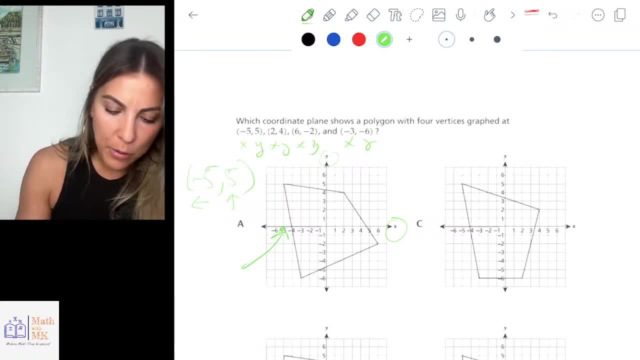 coordinate spot is positive. So I'm going to go up. So I'm going to go up one, two, three, four, five, And that puts me at this point, right here, that I've labeled. So I see that at least that point is correct. I'm going to look at the other answer choices to see if any of them don't. 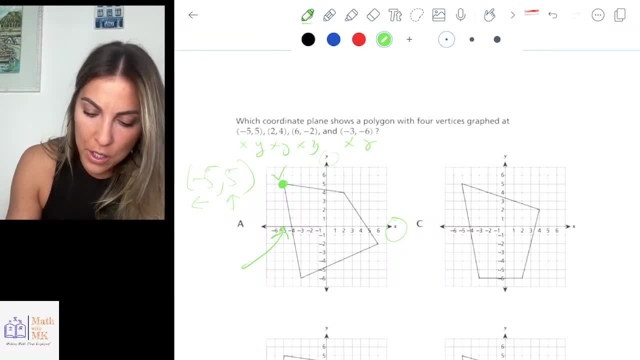 have that point, because then I can eliminate that answer choice. So choice C to the right has negative five, five, So that one looks good. Choice B at the bottom also has negative five, five. and choice D at the bottom also has negative five, five. So they didn't make. 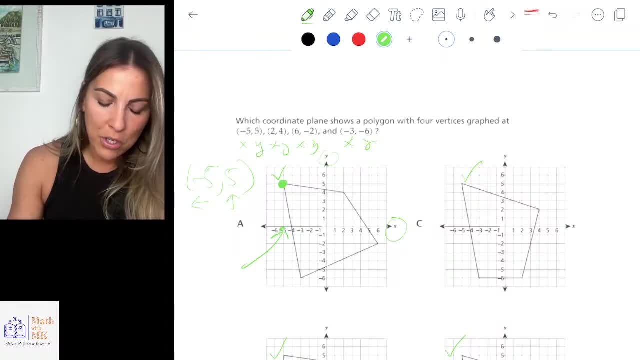 it that easy for me. We can't eliminate anything yet. The next order pair is two, four. Again, that order is super important: X, Y, X, Y. So the X is two. So that means that I'm going. 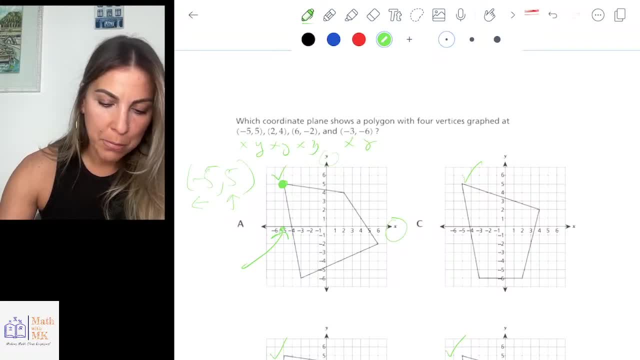 right. two spaces and then up four, which puts me at the red dot right here, Is correct in a. let's look at the other answer choices and see if we can eliminate anything. So if I move over to C, two, four, two, four would be right here. So it's actually not here, So C. 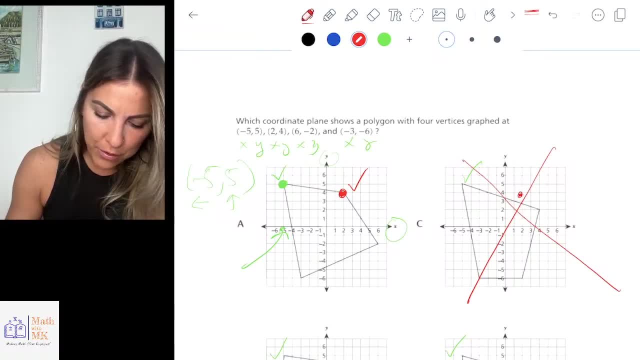 is out. Let's look at B. If I go to two four, there it is. So in B two four is good And in D two four is right here. So it's not on my polygon, So D is also out. So I've already made my. 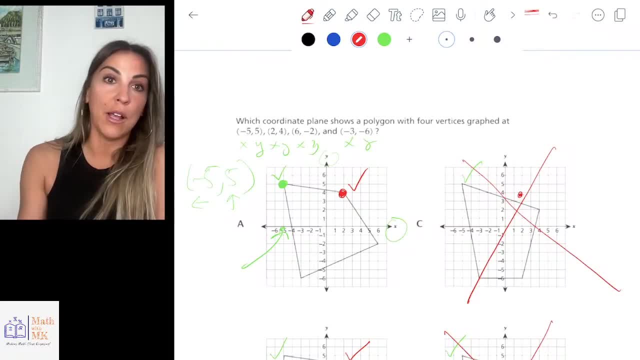 choice, my chances of getting this problem so much higher. Cause now we only have two spaces to work with, Moving on to six negative two, I'm going to go to the right six spaces and then down two, And that's going to put me at this blue dot right here. And if we 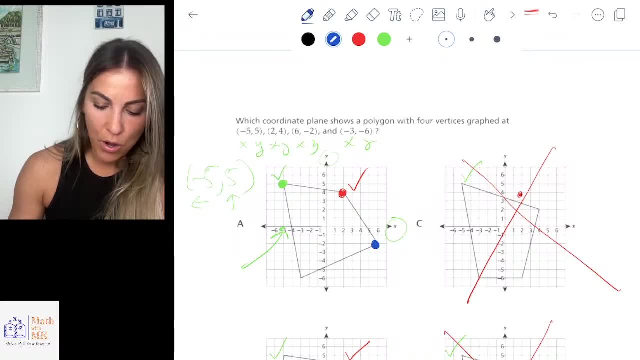 look at choice B: six negative two also exists. All right, So I picked the wrong order to go in because it's going to be the last one that determines it: Negative three, negative six. So we're going to go left- negative three and then we're going to go down to negative. 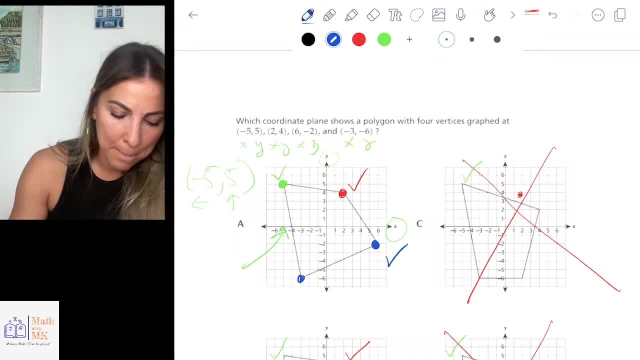 six. And that puts us at this other blue dot that I'm leaving, Which makes it look like answer choice is the correct choice. but just to be sure, let's look at choice B and make sure negative three, negative six is not there, So I go. negative three: I go. 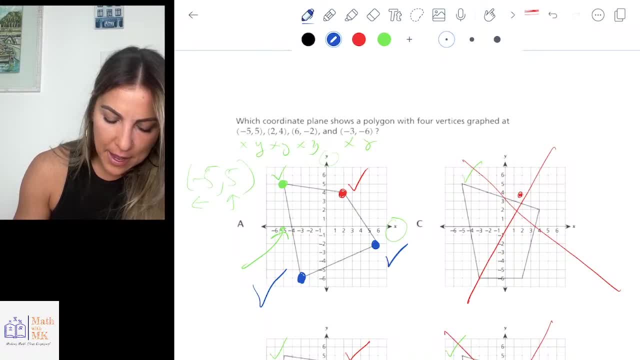 left to negative three, and then I go down to negative six. That point is not on that polygon. So choice B is also out and A is the correct answer. All right, So we're going to stop there for sixth grade problems and we will do some more next time that are in a different topic of.